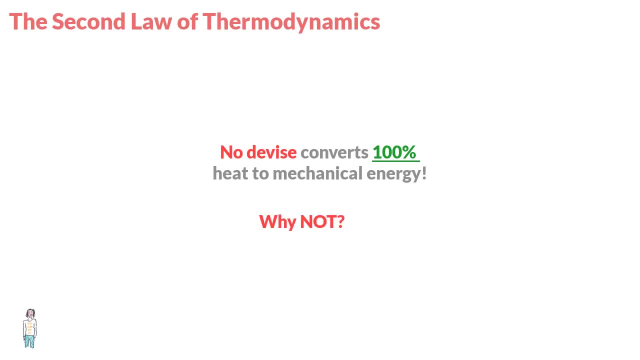 the question is: why not? Well, it's got to do with what physicists call the direction of thermodynamic processes And it is called the second law of thermodynamics. And as we move ahead, we'll get more clarity on what is the second law of thermodynamics And we'll also see 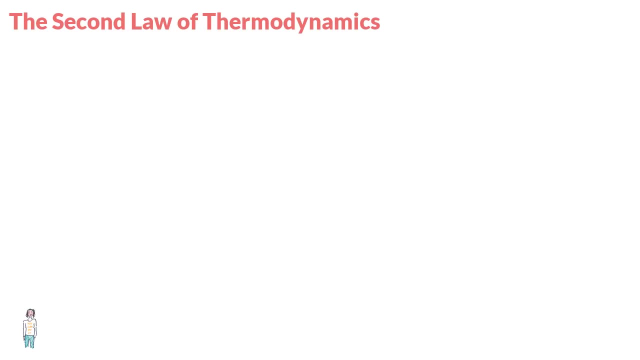 that this is probably one of the rare laws that can be stated in several ways, entropy being one of the ways of stating it. so let us study what the direction of thermodynamic process really means. now, all thermodynamic processes that you see in nature are irreversible, or in other words, these processes proceed in one. 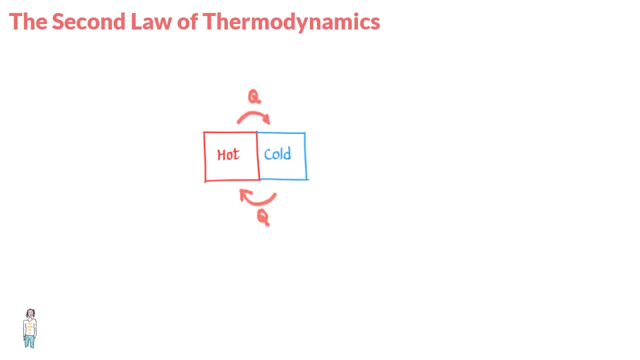 direction. only as an example that I've stated earlier. the flow of heat from a hot body to a cold body is irreversible. so is the free expansion for gas that we have studied in earlier lessons. now, sliding your mobile phone or a book across the table is also an irreversible process that converts mechanical energy. 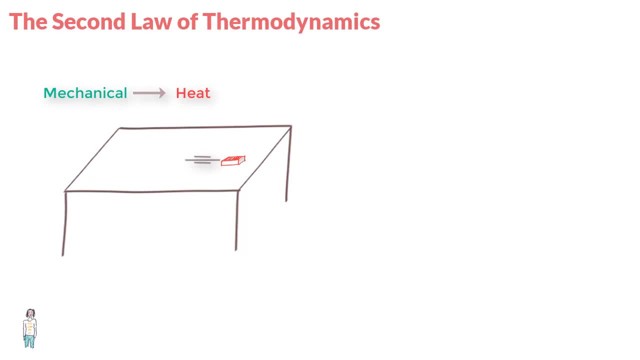 into heat due to friction. I mean, no one has ever observed a mobile phone sliding in the reverse and cooling down itself and the table. so it's. it's not a reversible process as such. or take a tire of a car getting deflated. by no stretch of imagination can you think of air from the atmosphere gushing into a? 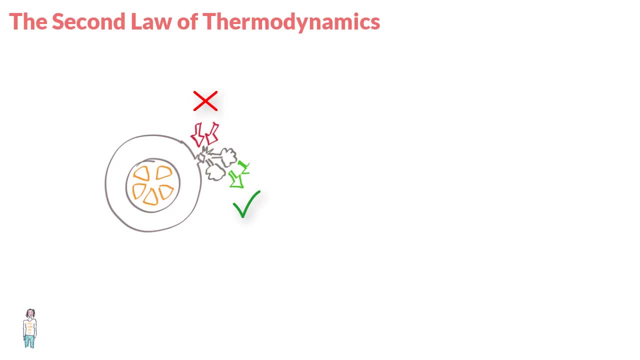 deflated tire. well, despite what you have said about every natural process being irreversible, there are some processes that could be termed reversible and we would normally say that these are idealized processes and we say that a system that can exhibit such an idealized reversible process is irreversible. 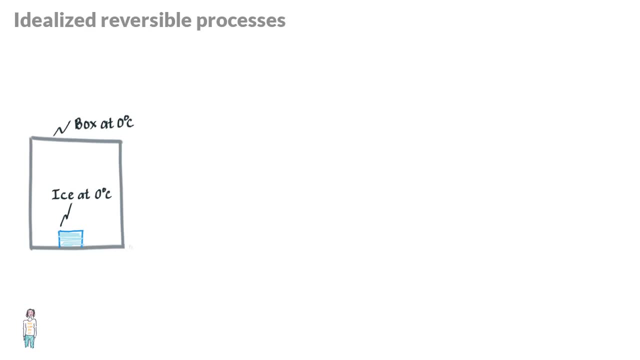 process will be almost in thermodynamic equilibrium. so this means that if it changed the state of the system, then any change that happens can be reversed by making some small changes that would be infinitesimal in nature to the setup. now the simplest example is that we can reverse a direction of heat flow between 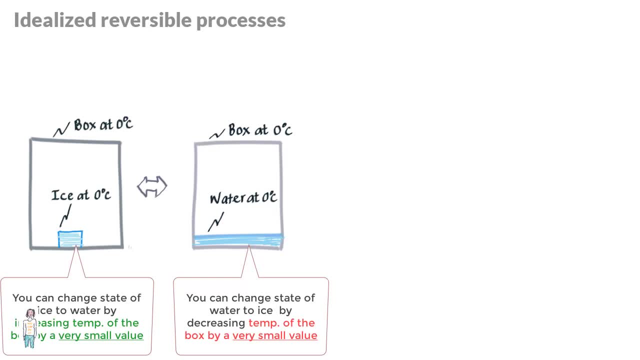 two bodies if the temperature difference is very small, and this can be done by making a very small change in temperature of either body. so the outcome of what I just explained is that all reversible processes should necessarily be in thermodynamic equilibrium. but then one can say that if 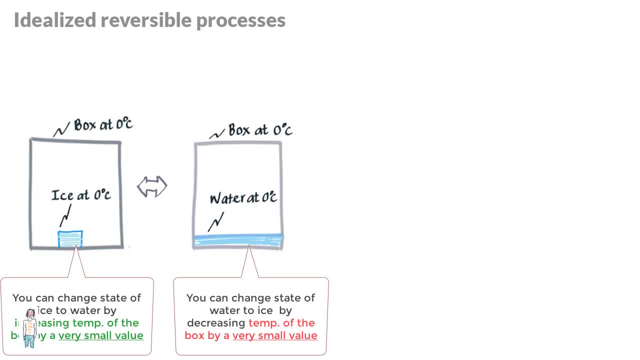 a system is really in thermodynamic equilibrium, how can change of state take place? in other words, heat should not flow into or out of a system if the temperature is the same across, and one would be correct in saying that, and that is the reason we say that. a 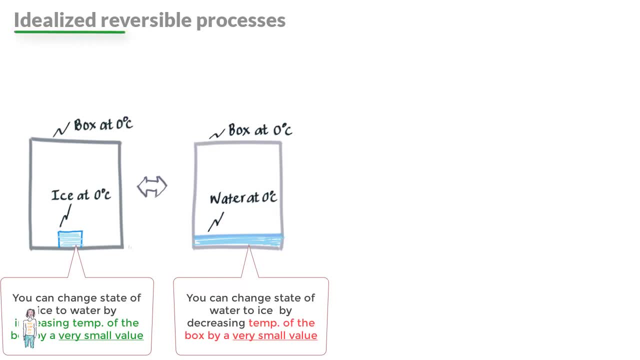 reversible process is an idealization that cannot be attained in the real world. but by making the temperature difference very small, we can make the system hover around the equilibrium state and in turn make the process almost reversible. and the moment the temperature difference becomes measurably large, the process becomes irreversible. 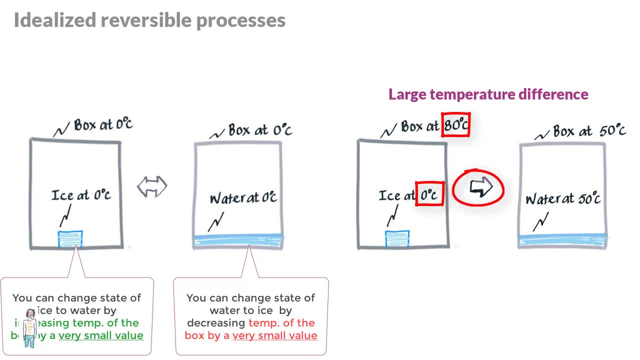 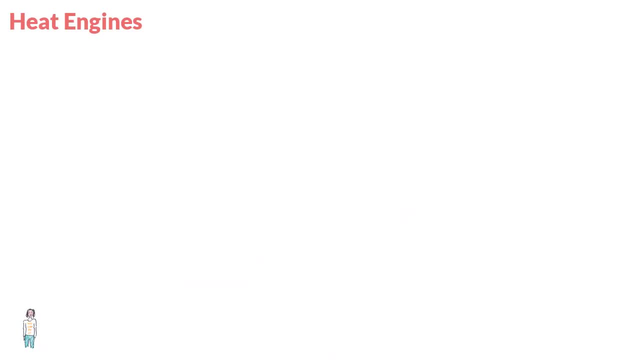 so let us take this discourse on the second law of thermodynamics forward by understanding what a heat engine is. well, a heat engine is any device that is capable of transforming heat into mechanical energy, at least partly, and this mechanical energy is also often termed as work done. in reality, what 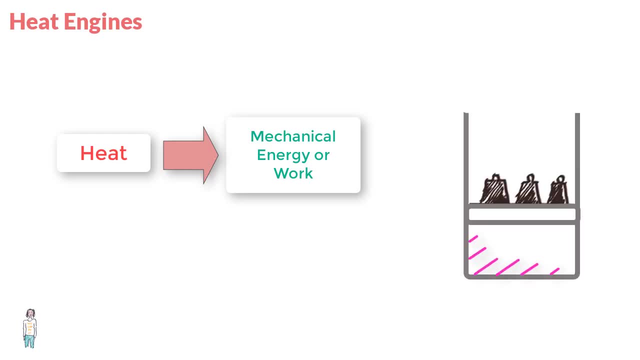 happens is that some matter inside the engine undergoes in flow and outflow of heat and, as a result, expansion and compression. now this substance is termed as the working substance of the engine and if you take, let us say, an internal combustion engine like the one you find in cars, the 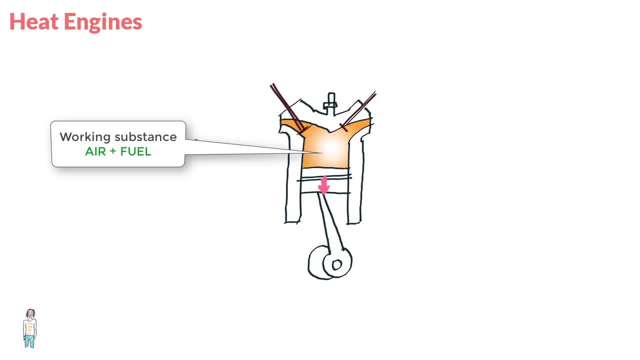 working substance would be the fuel and air mixture. so very often this working substance undergoes a cyclic process, which is nothing but a sequence of steps or processes that finally leaves a working substance in the same state where it started. So, while an internal combustion engine does not use the same air repeatedly, but we can still term it as a cyclical process, since the 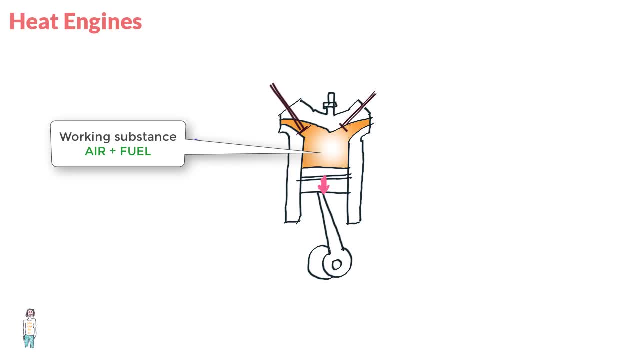 state of the engine at the end of the cycle is the same, even though new air is introduced in the engine. So typically a heat engine will absorb heat from a source that is at a measurably higher temperature, do some mechanical work and discard some heat at a lower temperature. For all practical, 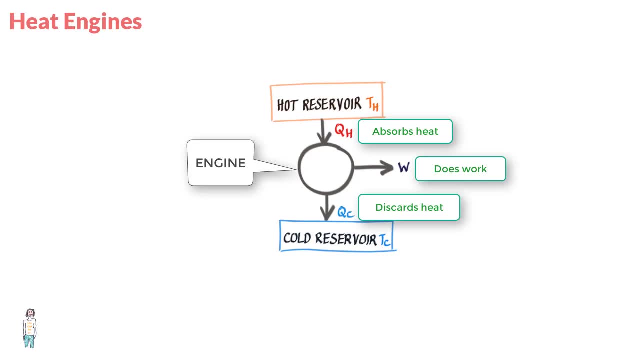 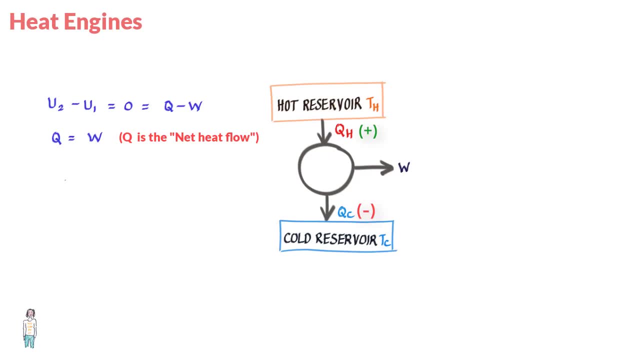 a system undergoes a cyclic process, its initial energy is lost. So when a system undergoes a cyclic process, its initial energy is lost. So when a system undergoes a cyclic process, its initial energy is lost. So when, therefore, W is equal to QH, but in real life this does not happen, because QC is. 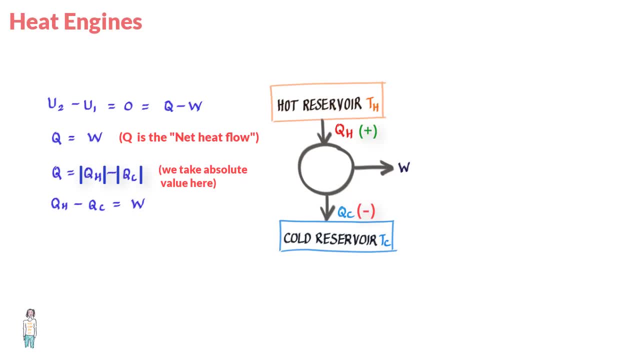 never zero, and therefore every engine has an efficiency measure which is E is equal to W upon QH. that is what most physicists like saying is: this is the ratio of what you get divided by what you pay for, and this is always less than one or hundred percent, which is what happens in real life too, and we can also 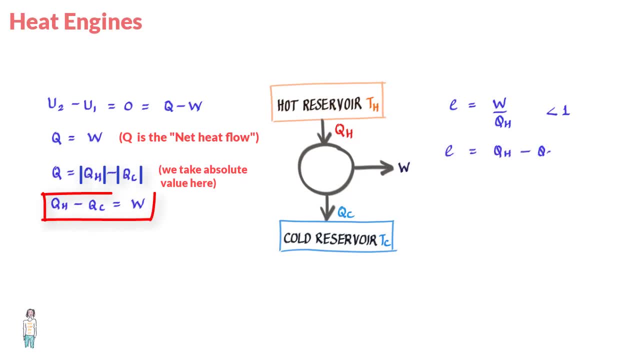 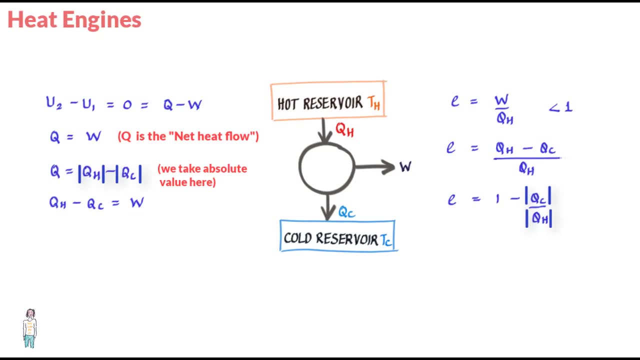 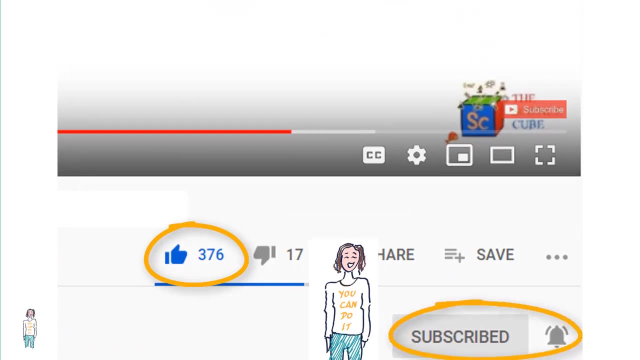 write this as QH minus QC upon QH, which is equal to 1 minus QC upon QH. so if you like this video, go ahead and give it a thumbs up, and please do not forget to subscribe to this channel for many more interesting videos. 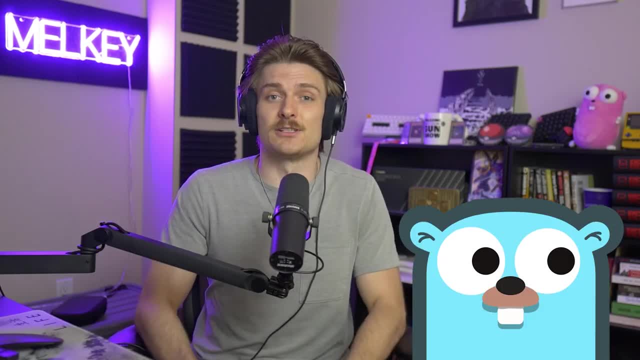 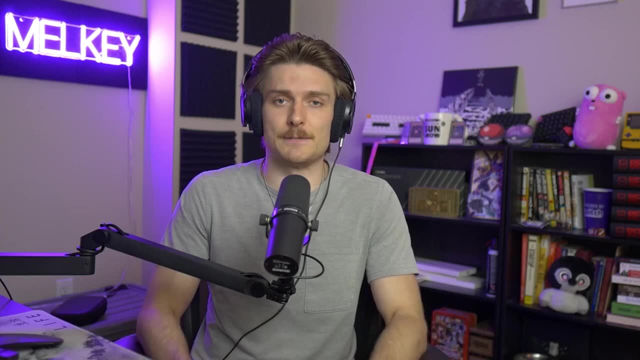 If you are coding in Go, you have probably asked yourself: what Go framework should I use? Now I want to be specific and focus on frameworks that people would typically use when they're building a Go backend for their API, and not so much frameworks they would use for creating. 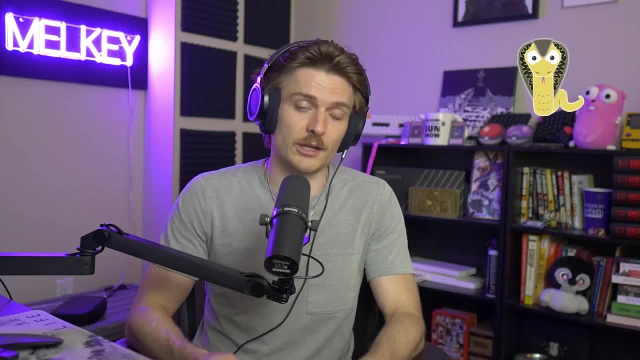 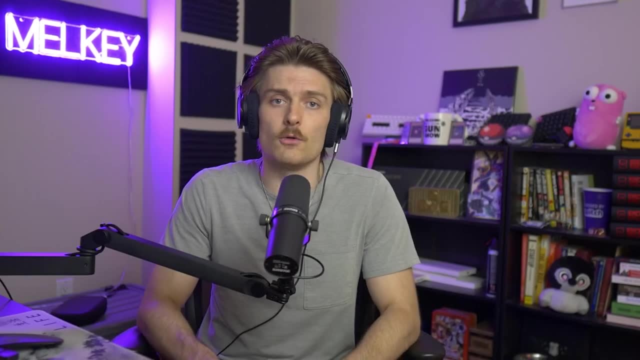 something like a CLI, which, if you haven't heard already, Cobra and Charm are great options, So go use them. It doesn't take a whole lot of effort to do one quick Google search on what Go framework to use to see a whole bunch of lists pop up, and then you get yourself into what I like. 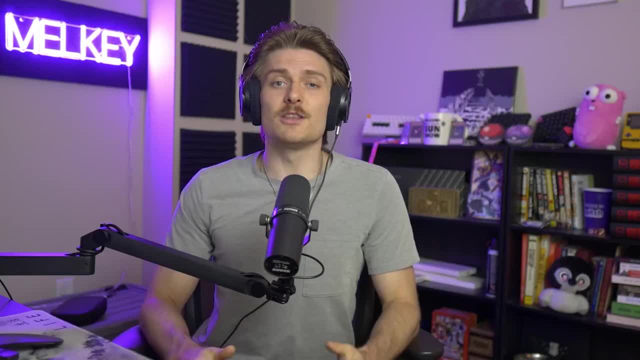 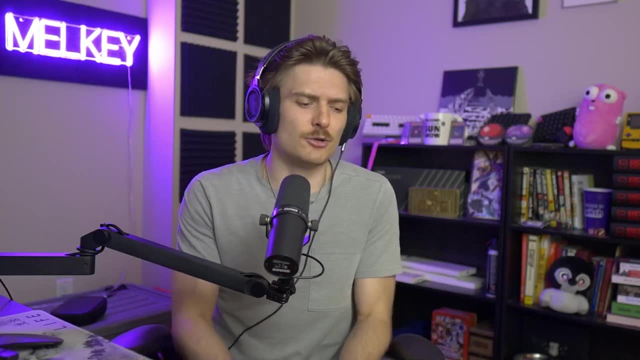 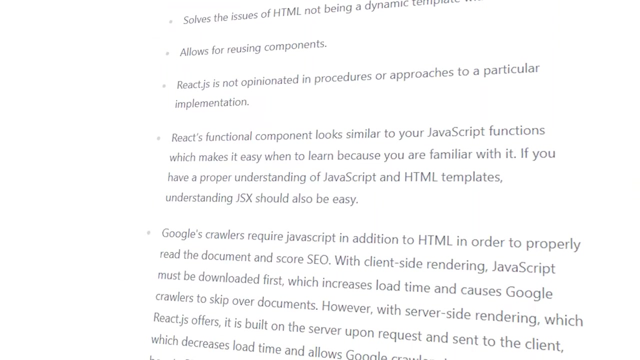 to call the JavaScript problem. The JavaScript problem is when there's too many options of what tool library framework to use, without actually knowing which one you truly need and want for your applications. In JavaScript there's React, Vue, Svelte, Solid Astro. Next. I mean it's. 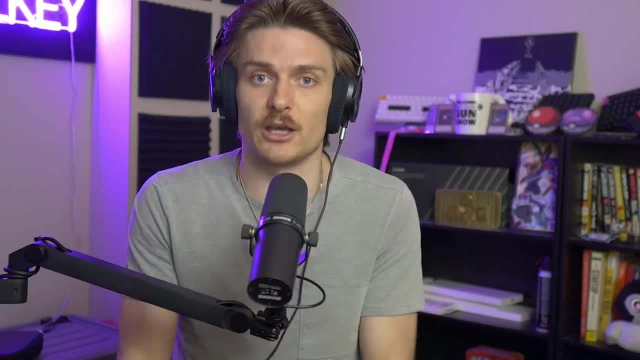 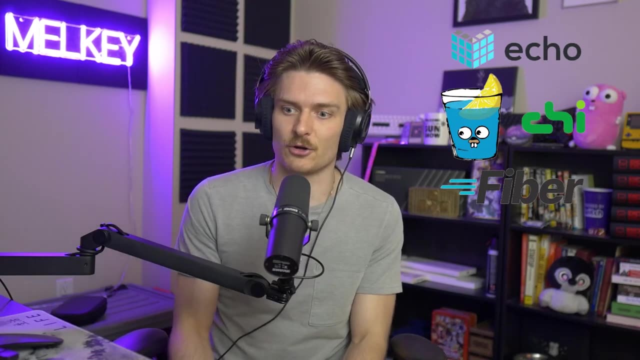 JavaScript. The ecosystem is evolving and changing every single day, But in Go, I mean, there's also a lot of options. There's Djinn, there's Chi, there's Fiber, there's Echo, there's Vulpix- That's a Pokemon. I try to trick you. 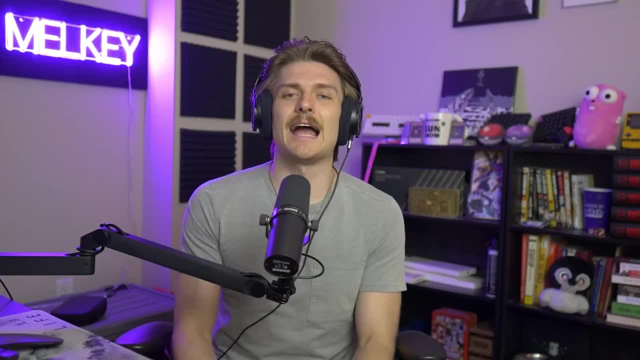 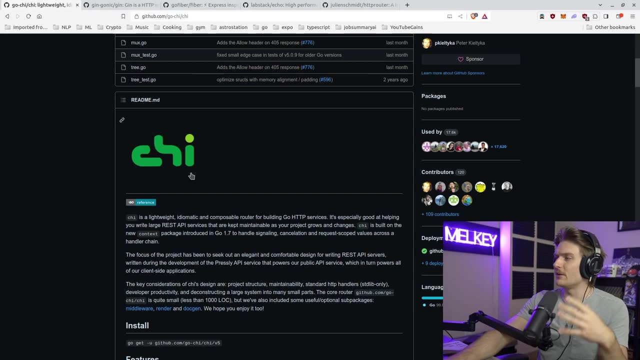 Which framework is right for them? Well, that's the actual thing. There is no right framework in Go. So you can see, here I'm on Go Chi And if I just read the first bit of the readme, Chi is a lightweight idiomatic and composable.